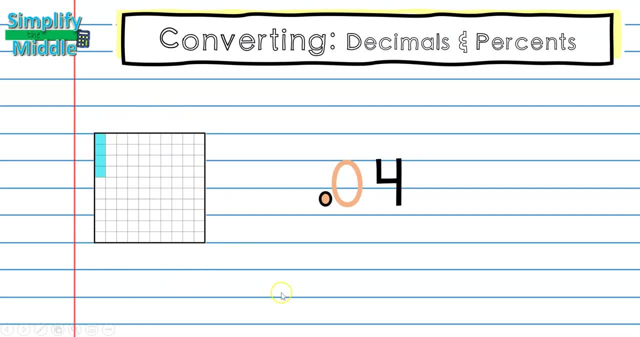 in the term of hundredths, I can see I have four pieces shaded. Let's look back at this example again. I remember that this is 40%, so that means that 40 out of 100 pieces have been shaded. I could divide 40 by 100.. 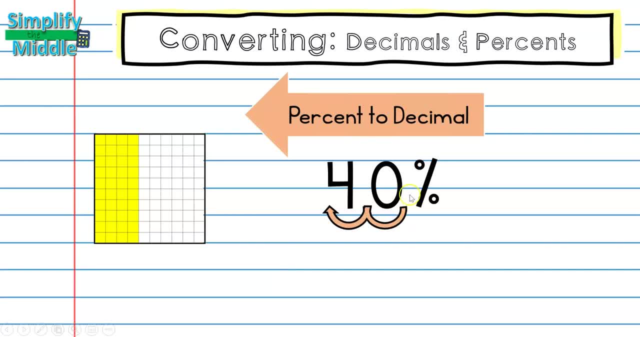 The faster way of doing this is moving our place value two places to the left. I'll add my decimal and drop off my percent sign. Now think back to the blue 4% We ended up with. 4% was a decimal of four hundredths and 40% is a decimal of four tenths or 40 hundredths. So there is a very big. 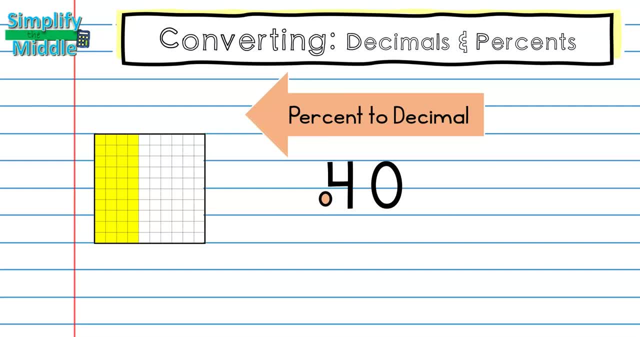 difference. We have to make sure that we are moving our decimal, the correct number of places. if we are going to use that method, Let's try another example: 93%. Pause the video and see if you can do this one on your own. So what we have here is our 93%. We're going to move. 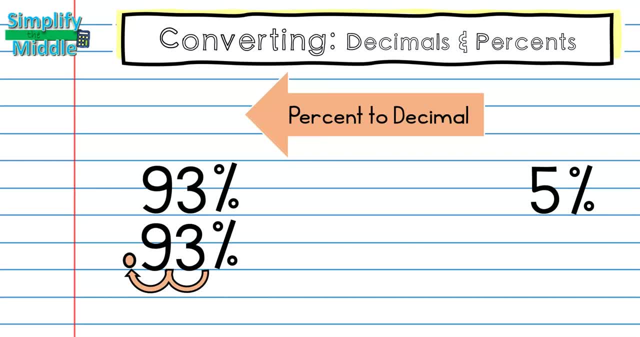 our decimal place, two places and we end up with 93 hundredths. Did you get that one right? If you did, let's try 5%. On this one, I had to add in a zero for my place value, So this one is 5 hundredths. 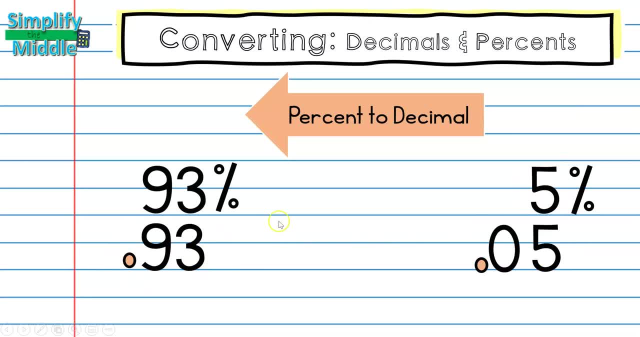 is the same as 5% and 93 hundredths is the same thing as 93%. So we could imagine this grid has 93 of those boxes shaded and this grid only has five of those boxes shaded, not even a full column. 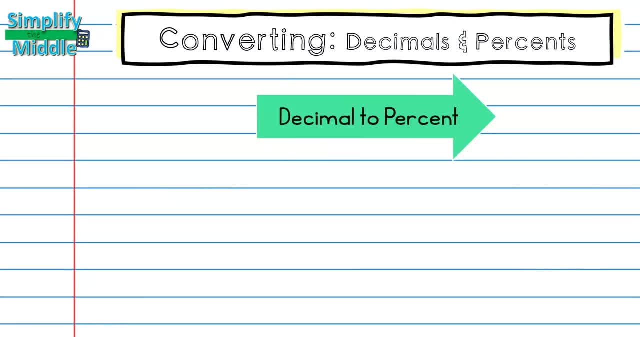 We also can go the other direction, from decimal to percent. As you can imagine, it's the same principle. This time, instead of dividing by 100, we're multiplying by 100. So we can move two place values to the right. This time we'll be moving our decimal over and drop in adding on a percent. 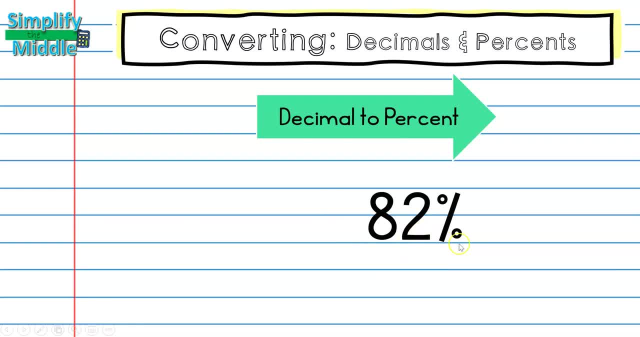 sign. My decimal is still here. I just haven't written it because there's nothing following the decimal, So I can assume that this 82 is 82 point. if you were confused about where the decimal is going, Why don't you try Pause the video?